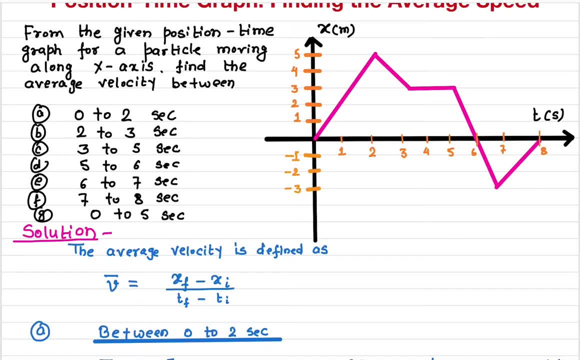 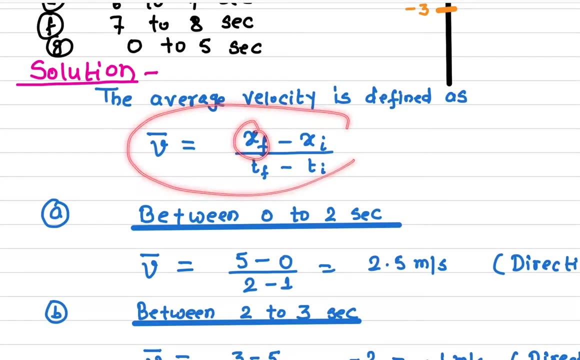 find out the average velocity. what we need to find out is the average velocity between the is the position, the final position, the initial position and the time difference. so the way it is defined, the average velocity is xf. what is f stands for the final position and this is the initial position. that's. 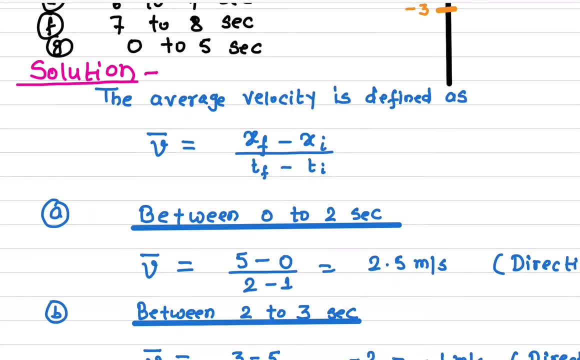 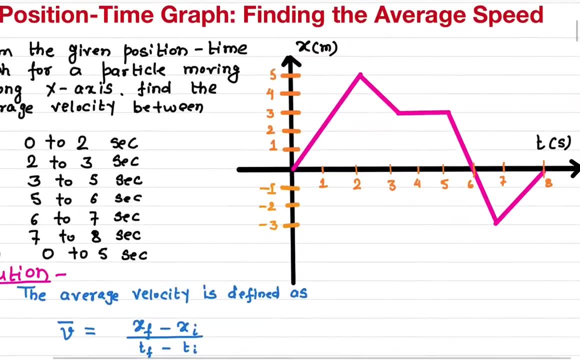 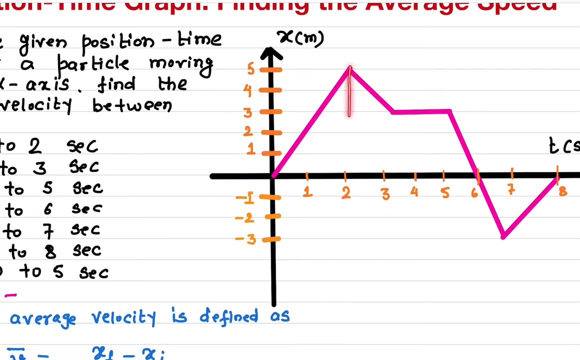 the final time and this is the initial time, so we need to know the position, okay, so let's first calculate between 0 to 2 second, or in this range here, between 0 to 2 second here. so at time, two t equals to two second. 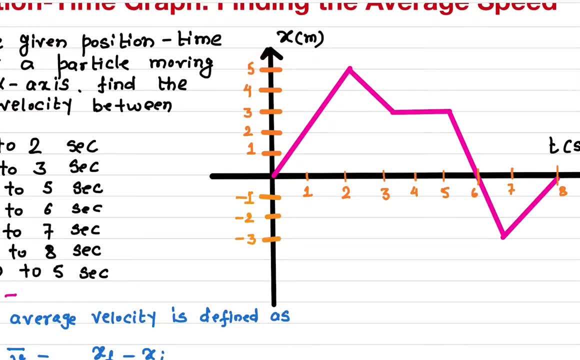 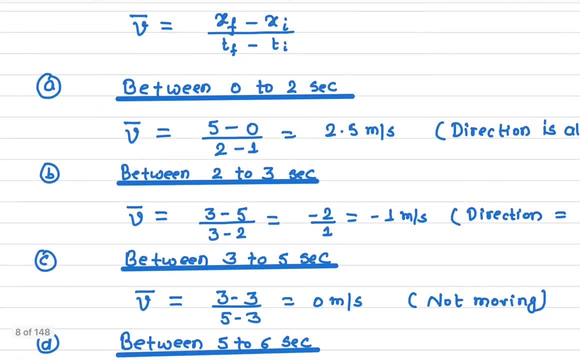 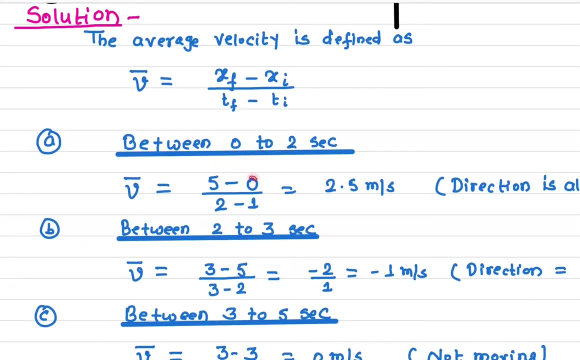 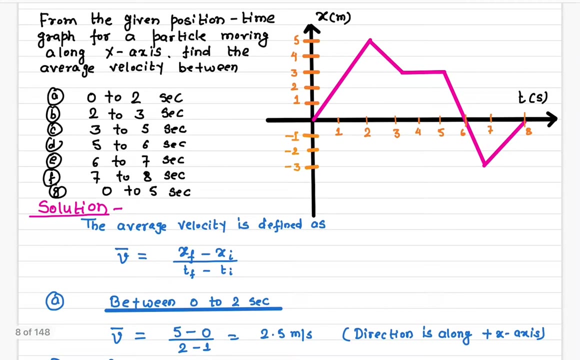 what is the position? the position is five, and at time t equals to zero. what is the position? that is zero? so just plug in in this equation: at time equals two. second, the position is five, and at time equals to zero. second, the position is zero. so you see, now you click, you can clearly see here from this graph: so this is the final position at. 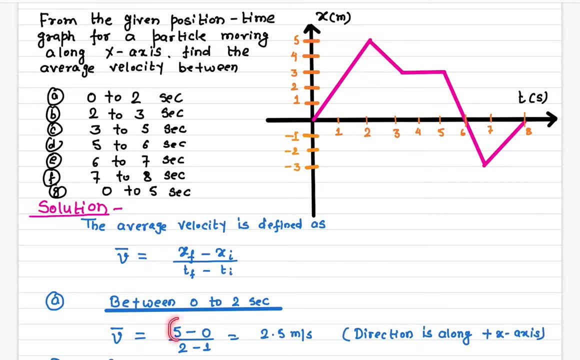 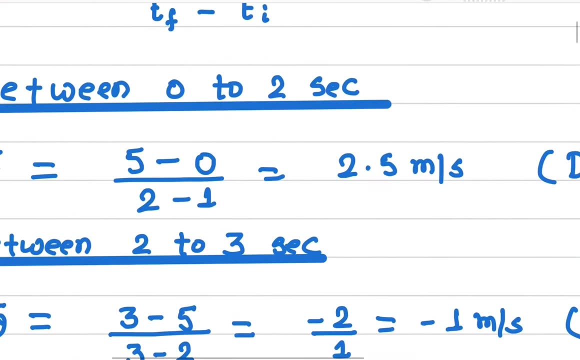 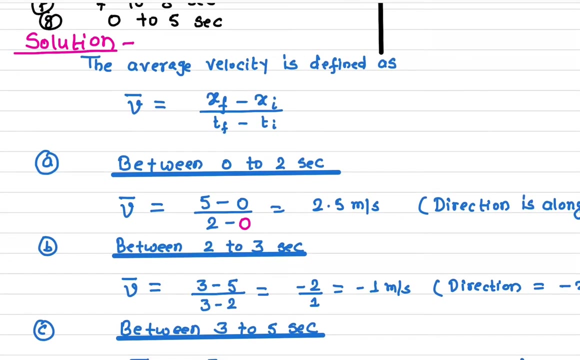 time. t equals to two second and this one is five. so just plug in five and time equals to zero. what is the position here? this is zero and this time is two minus. it should be zero here, okay, so i'm just making small correction here, although mathematically it is correct. 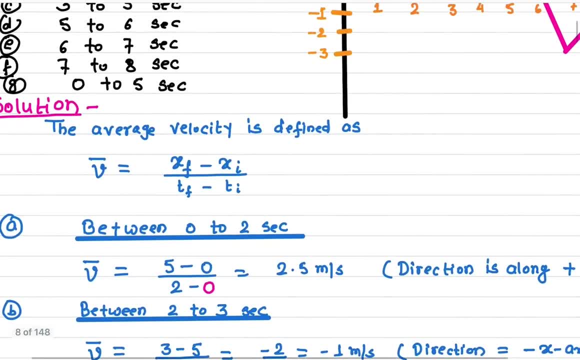 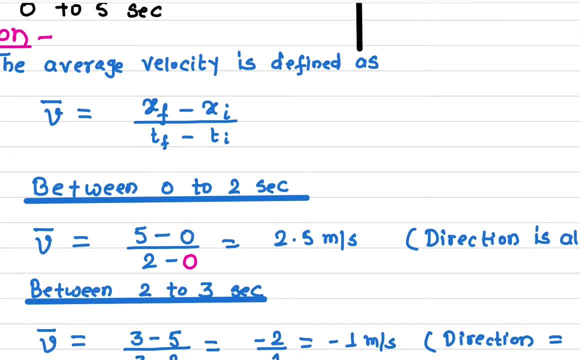 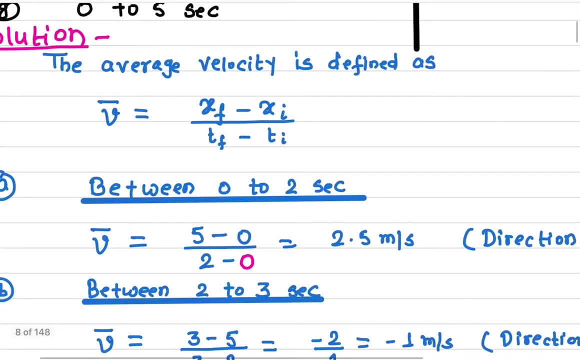 so five over two is 2.5 meter per second. so this quantity is positive. what does it mean? that means the particle is moving along the positive x direction. okay, so it is moving along a positive x-axis and with an average velocity of 2.5 meter per second, and you can also: 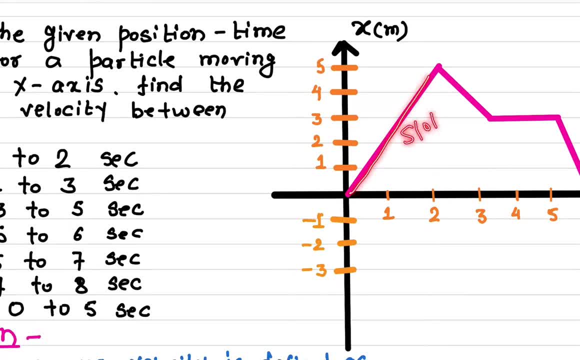 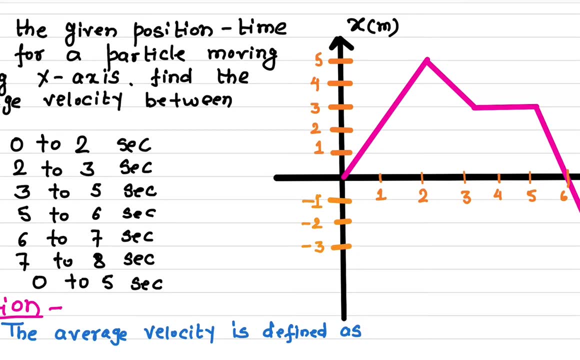 see from this graph the slope. the slope is positive. whenever the slope slope is positive, that means the particle or the object is moving in the positive direction. okay, and now let's find out what is the average velocity in this interval, in this time interval, and you can immediately see that the slope here is negative or it is downhill. this is the 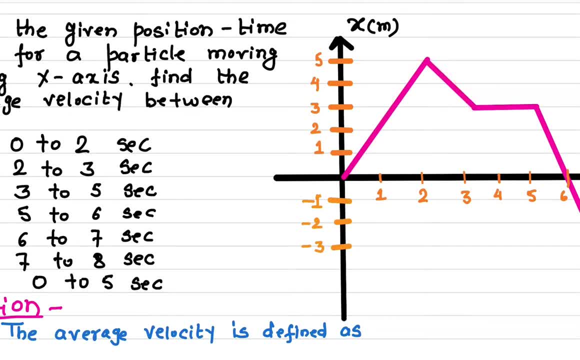 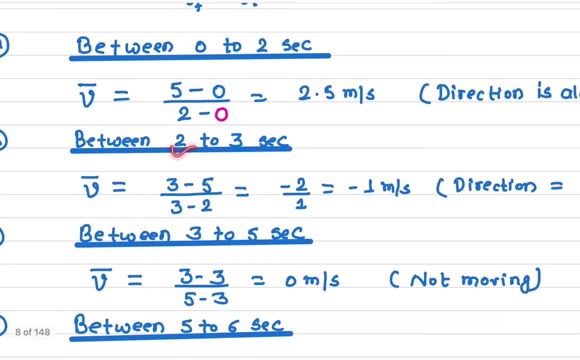 uphill and this is the downhill. the downhill means the slope is negative. what does that mean? that means the average velocity in this case has to be negative. now let's calculate this one. so again, between two to three second. so what do we have? what we need to find out? 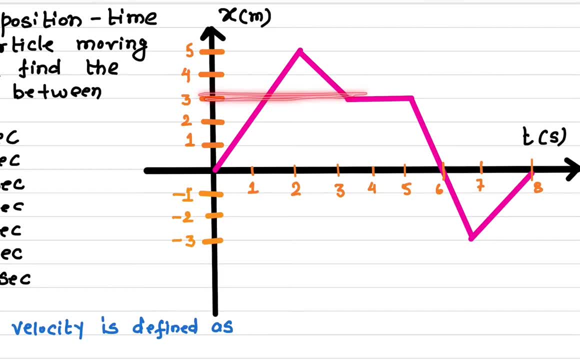 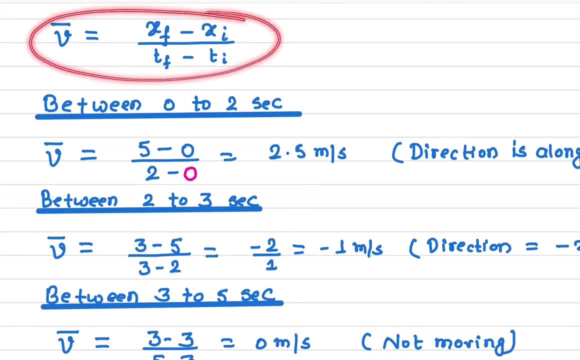 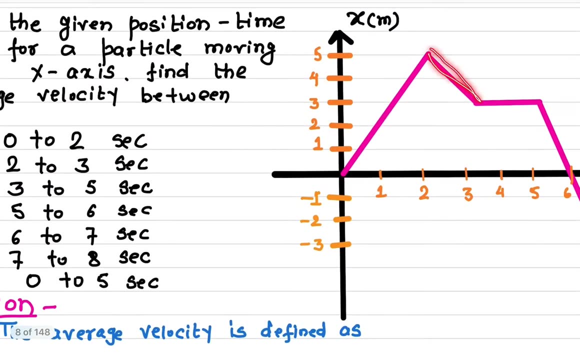 what is the position at this point? that's the final position. the final position is three second, so that's the final position. so i'm just plugging into this equation here: the final position is three second, and the initial position, because we are interested in calculating in this interval. 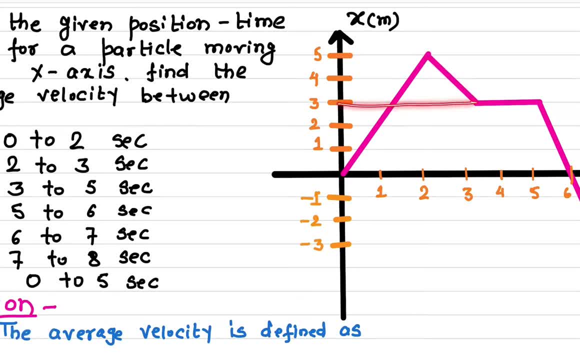 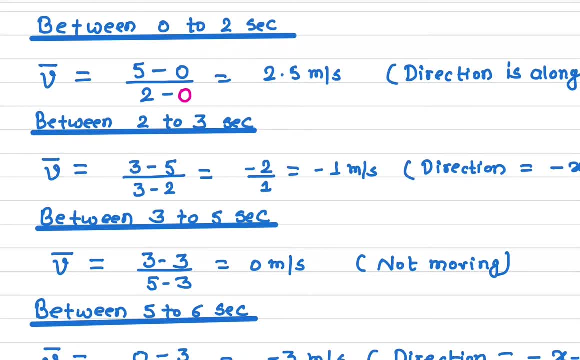 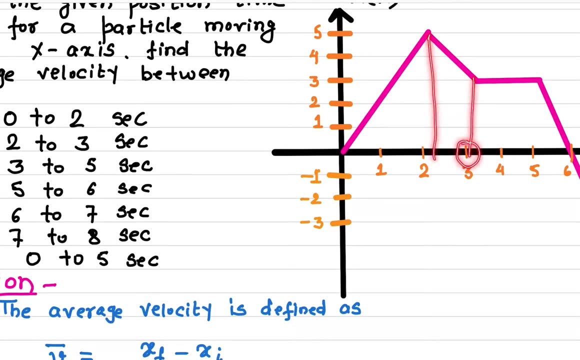 so the initial position is five and the final position is three. so that's all i'm plugging here: three minus five, and the time is three second and two second. you see, now we are interested in finding out this here. so this is the final time. this is the initial time: three minus two second. 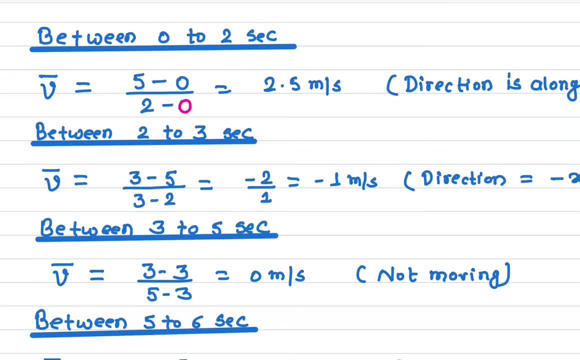 and if we solve it, then it will be negative two divided by one, which is negative two meter per second. again, minor correction here. okay, so what does this mean? the negative sign tells you the particle or the object is moving in the opposite direction. okay, so it was first. in this case it was. 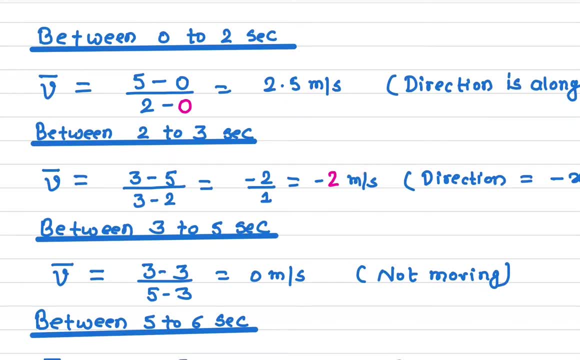 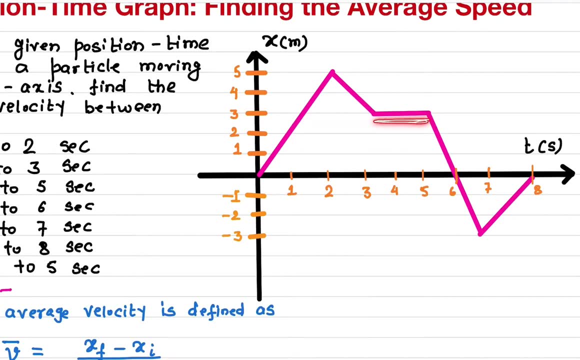 going forward and now it is coming backward. that's what it means. now let's calculate from three to five second from here, from this range here: three to five second. so what is the final position at this point? at this point, the particle, the position of the particle, is three, and even at three time, 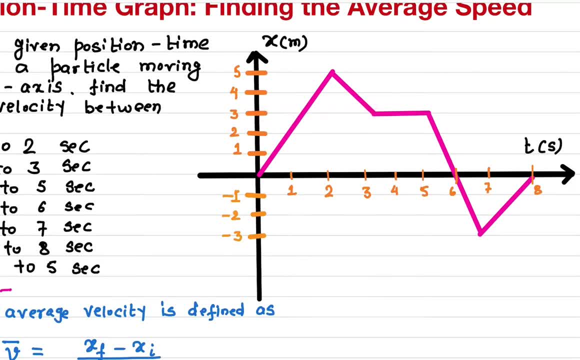 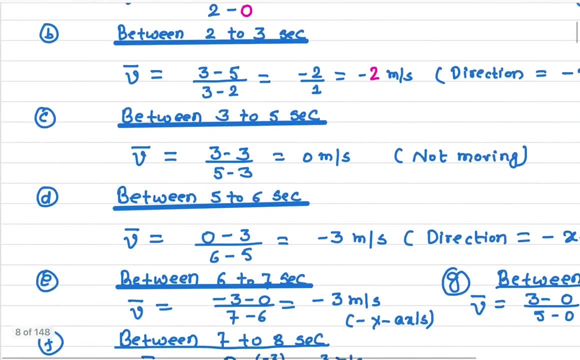 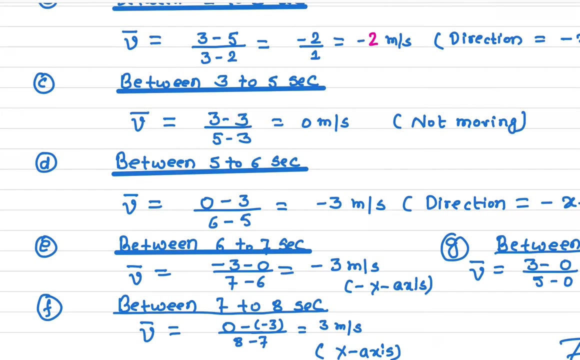 equals to three. second, the position is three. second, what does that mean? the particle is not moving at all. there is no change in position between three to five. second, the position is not changing, so that means the particle or the object is at rest. so i have calculated here. so the final position is three and the initial position is three. 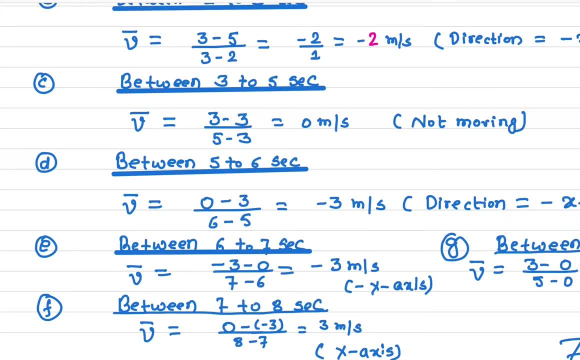 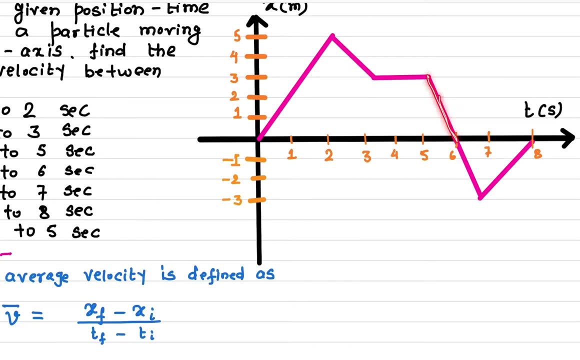 which is zero meter per second. that means the particle is not moving at all. so now we calculated in this range now, let's calculate it in this range now, and what you can immediately tell you from this one is: there is a downhill, more downhill. okay, downhill means 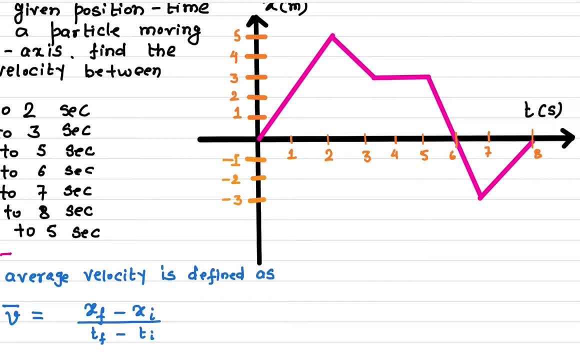 there's, the average velocity has to be negative. so what is the final position at this point? the final position at time equals to six. second is zero, and the and the initial position at time equals to five. second is three. so let's plug in in this equation here between five to six seconds. 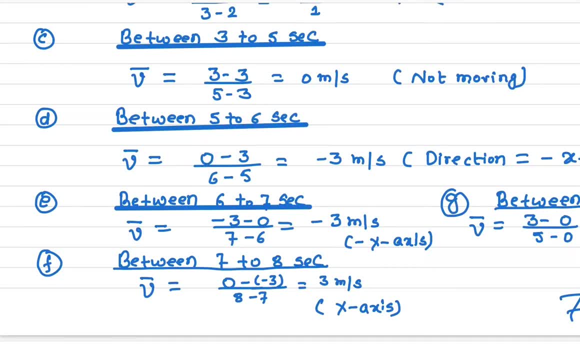 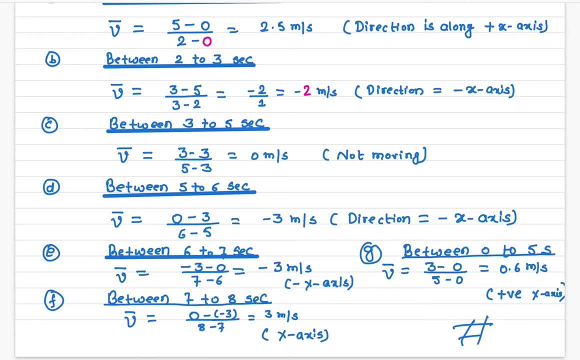 at time close to six. second, the final position is zero. at time equals to five second, the position is three and this is the times 6 minus 5. what i get is negative 3 meter per second. the more the downhill is or the uphill is, the higher the average velocity is. 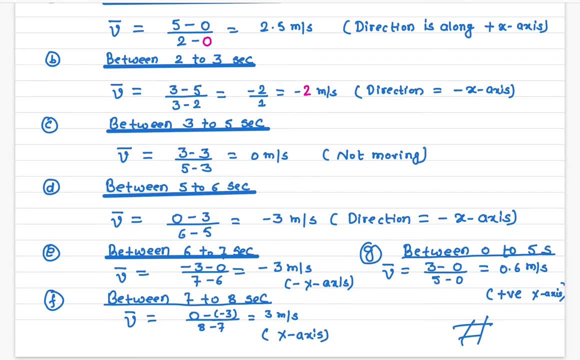 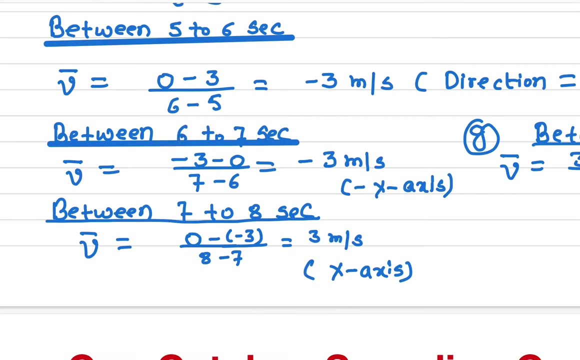 so when you solve it, what you get is negative three meter per second, and the negative sign tells you the particle is moving in the negative x-axis. and now I'm not going to solve this, this here again. the same way you can calculate from six to seven, second. from seven to eight: second. let's do this one from seven. 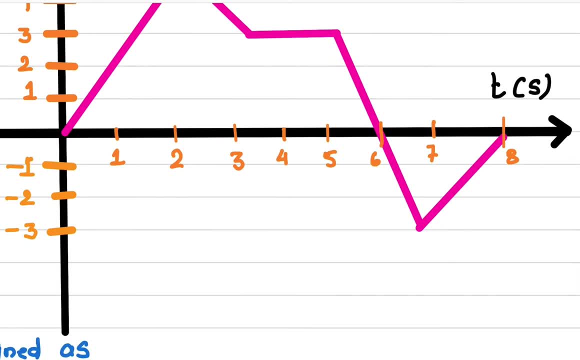 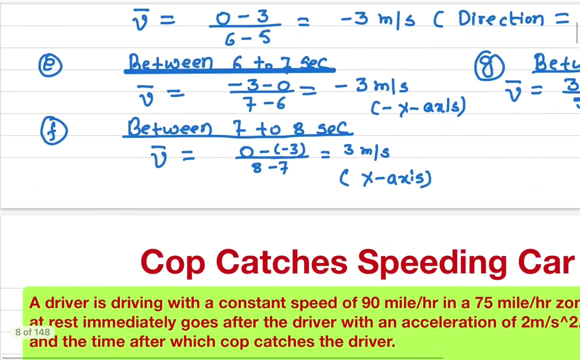 to eight second, seven to eight second. between this time, what is the position at this point? the position at this point is zero. what is the position of the particle at time? equals to seven second. this one is negative three. so you have to write down the negative. so once we do that now, let's see here. so at time. 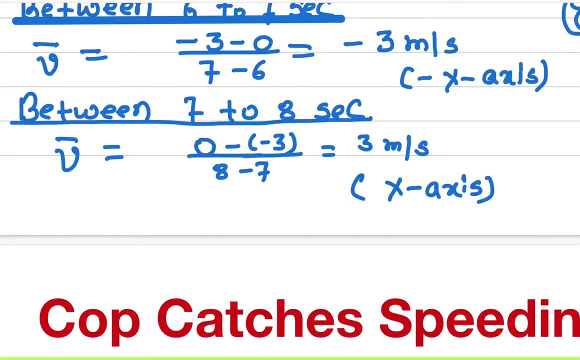 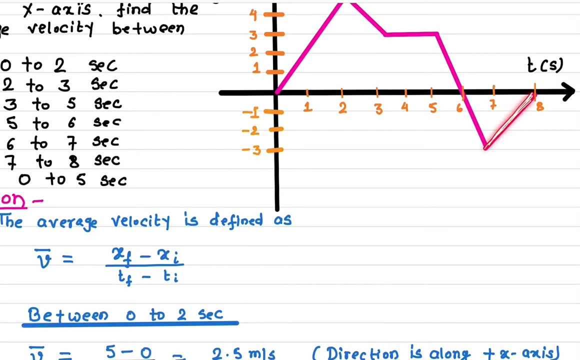 equals to eight. second, this is the particle is at zero position, negative and at time equals to seven. second, the particle position is three. so this negative and this negative will make it positive. so this is three meter per second now. okay. so what does this mean? that means in this case, the particle is moving in the forward direction. okay. 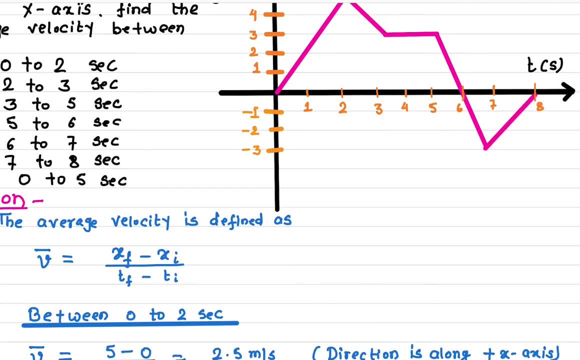 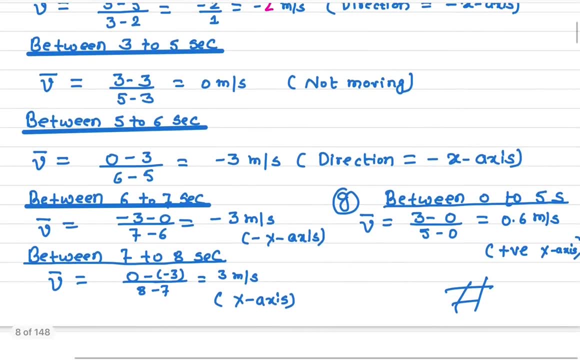 because this is an upward slope. that means the particle must be moving in the forward direction and the particle is moving in the upward direction and the particle is moving in the forward direction or the positive x-axis. the same way, now we can calculate from zero to five second. so this is zero and this 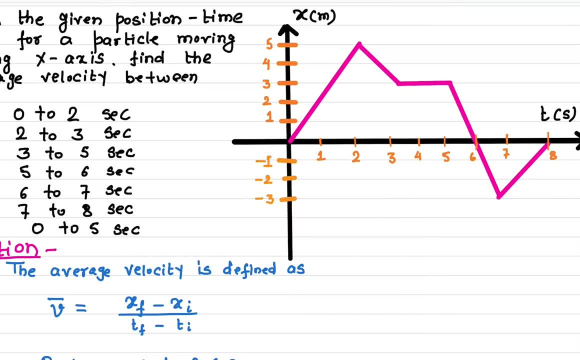 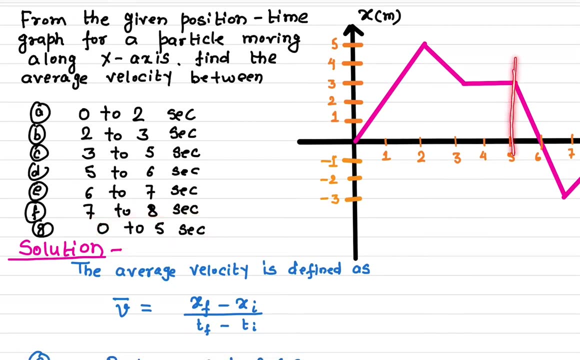 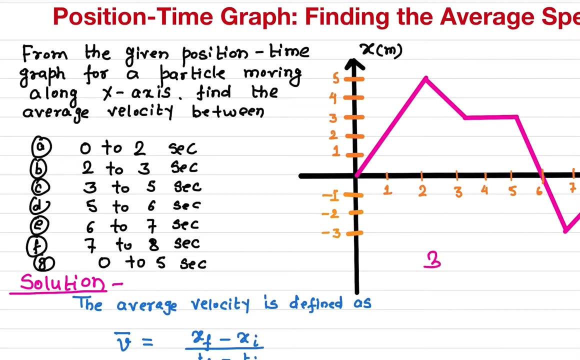 is a five second here. so how did you calculate the average velocity between these two? time again, the information you need is the position. so between zero to five second here I'm solving for this now. so at time equals to five second. the position is three, so three- let me write down here three- and at time equals. 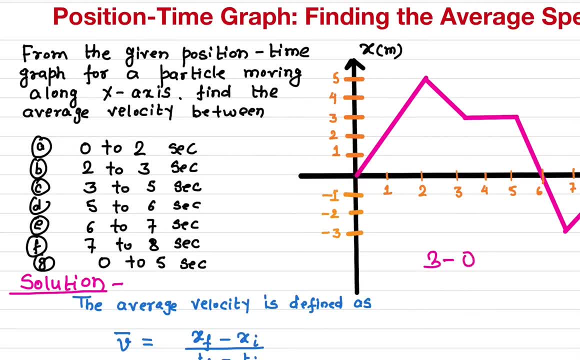 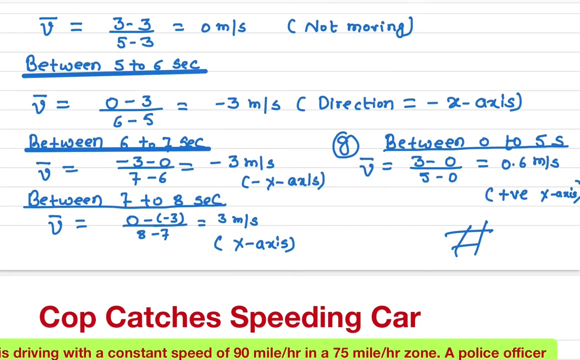 to zero second. the position is zero divided by the time. the time at this point is five minus zero, so three divided by five. if we solve it, it will be 0.6 meter per second. that's what exactly I have solved here: 0.6 meter per second. and it is still moving along the positive x axis. okay, so. 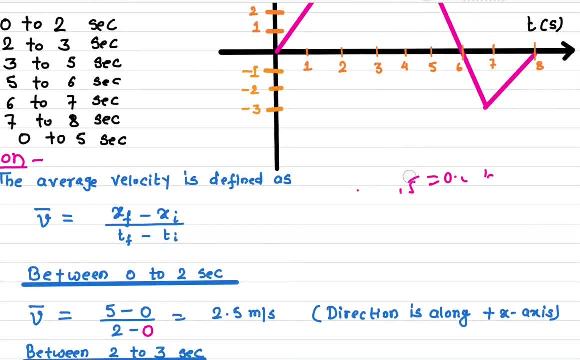 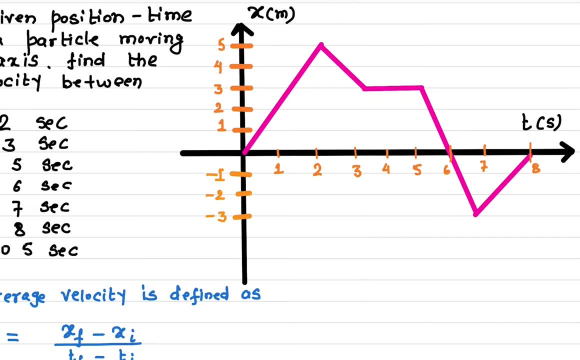 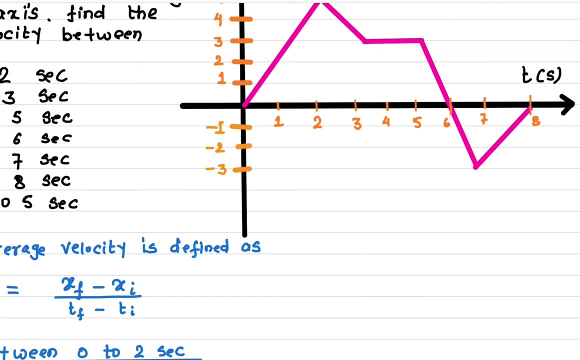 that's how you find the average velocity from a given position. time graph. all right. so if you want more interested, let me draw a more picture of this one. so now let's say: let's say how is the particle moving? let's say I'm drawing here, this is the x-axis and this is the position of the particle moving. so I'm 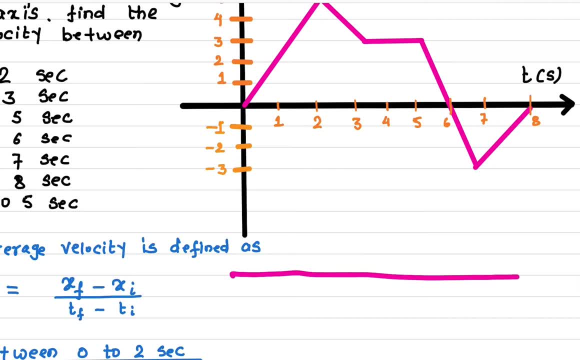 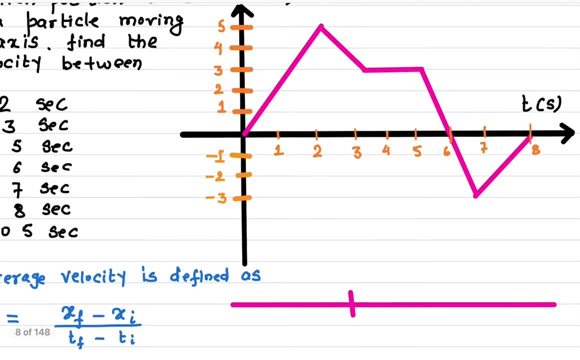 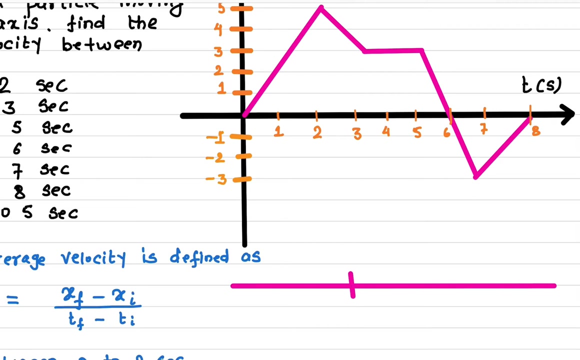 x-axis and you were initially at this point. so let's say how you moved. so first, you moved from zero to five meter, in time equals to two second. so first, what you did? you moved five meter. you moved five meter. so this is the first motion here. 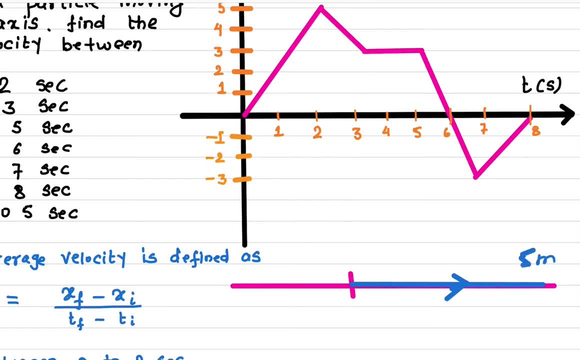 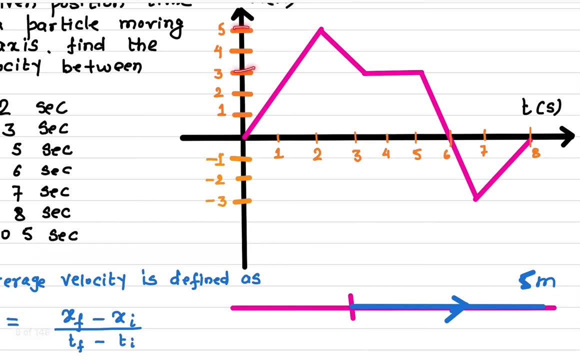 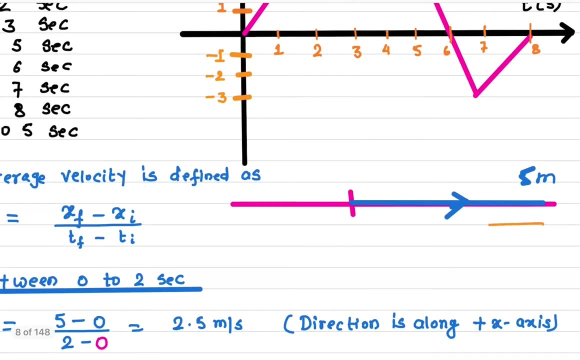 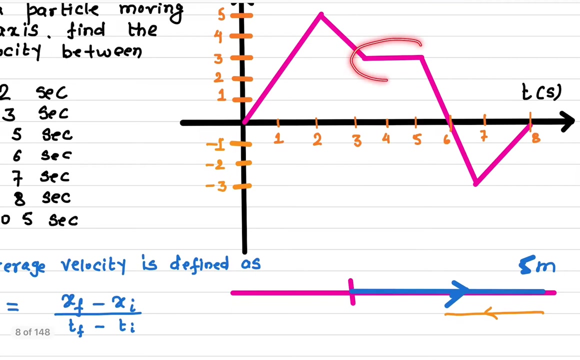 okay, this is the five meter, five meter. and then what it did? you moved backward. how much you moved? you moved from five meter to three meter in the backward direction. so your second motion is five meter two. you move this way. okay, and then from in this interval, you: